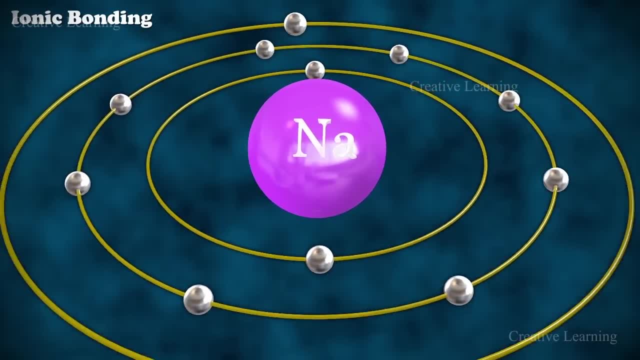 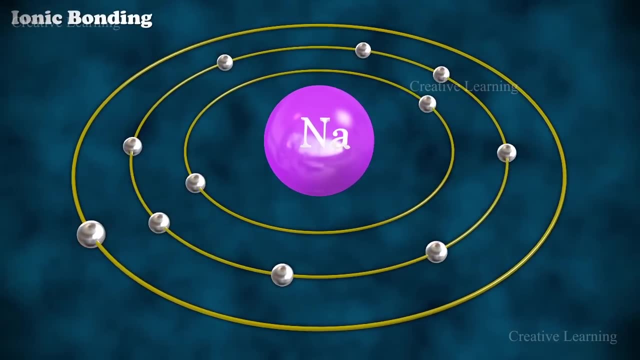 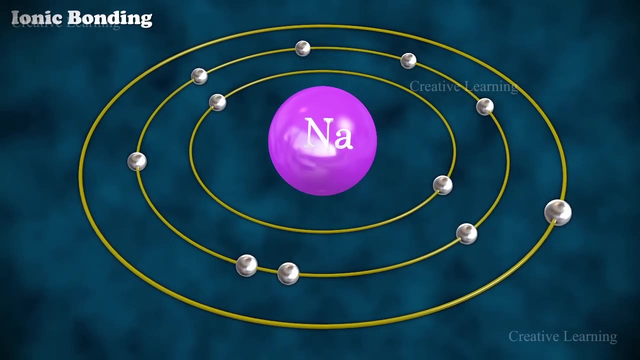 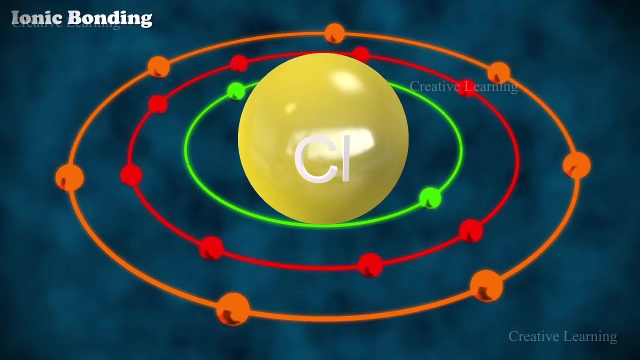 rule. Sodium metal has electronic configuration as 2,, 8 and 1.. It has one electron more than a stable, noble gas structure. If it gives away that electron, it would become more stable. On the other side, chlorine has electronic configuration as 2,, 8 and 7.. 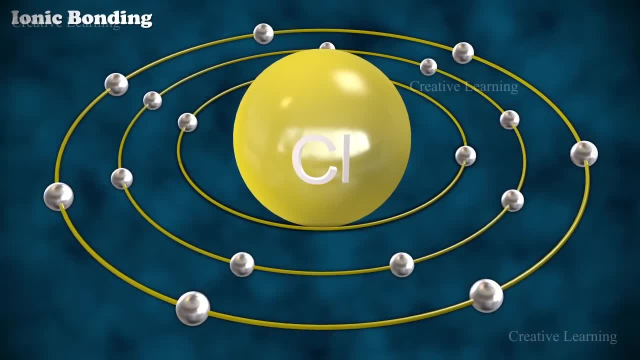 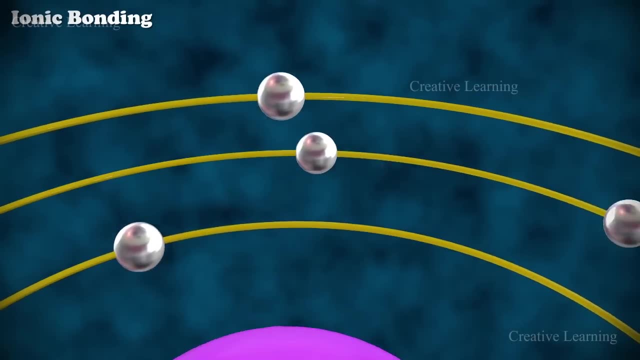 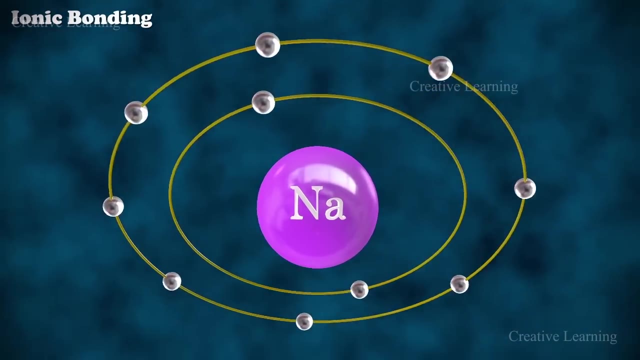 It has one electron short of a stable, noble gas structure. If it could gain an electron, it too would become more stable. Thus the sodium atom donates its valence electron to achieve stable octet configuration. This creates a positively charged cation due to the loss of electrons. 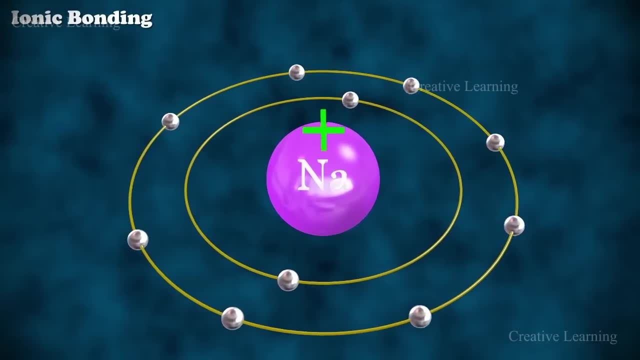 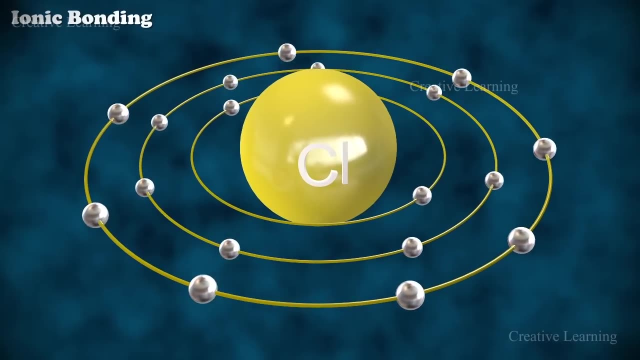 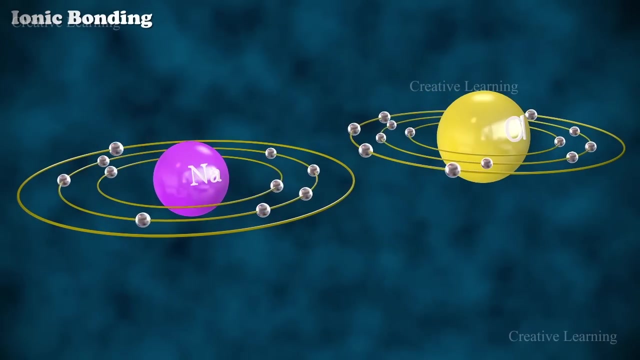 The electron is then transferred to the valence electron. The valence electron is then transferred to the octet electron. The chlorine atom receives one electron to achieve its stable octet configuration. This creates a negatively charged anion due to the addition of one electron. 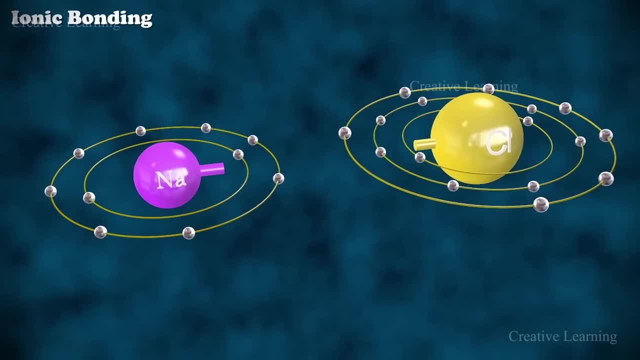 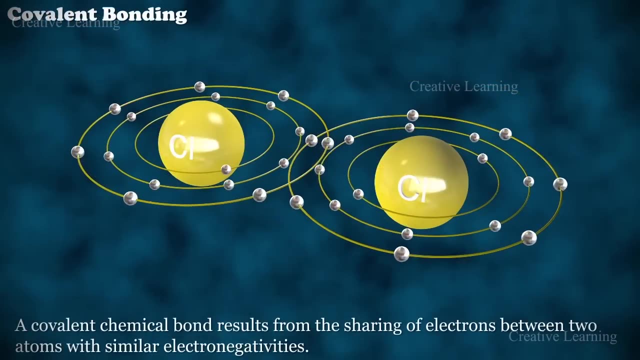 The sodium ions and chloride ions are held together by their strong electronic attractions between the positive and negative charges. Covalent Bonding. Covalent Bonding is a covalent bond. Covalent Bonding is a covalent bond. The covalent bond is an analogouse makenh discussion. 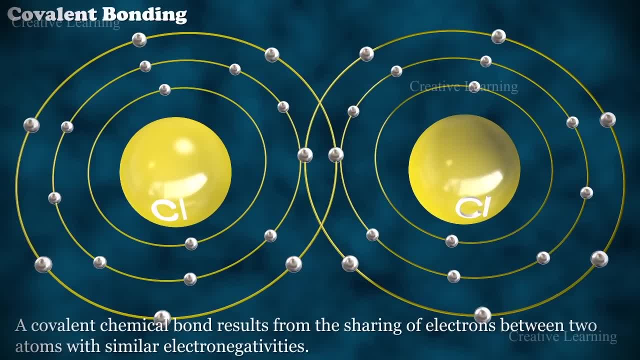 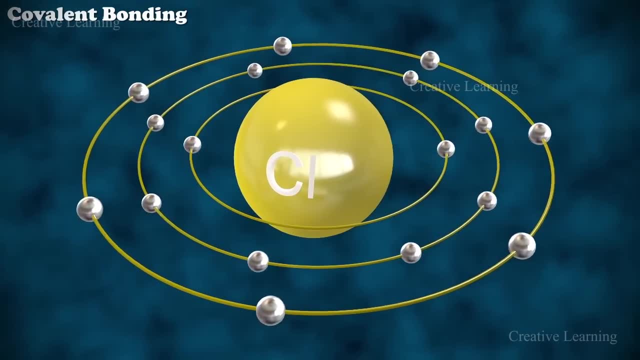 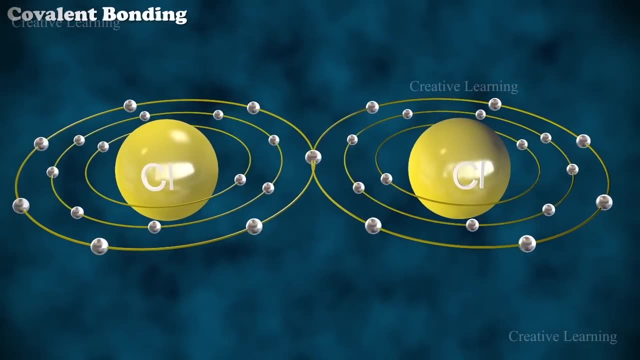 Covalent bond is a covalent bond. Covalent bond results from the change of electrons between two atoms with similar electronegativities. Electronic configuration of chlorine atom is one electron short of the argon configuration. The formation of the chlorine molecule can be understood in terms of the sharing of a. 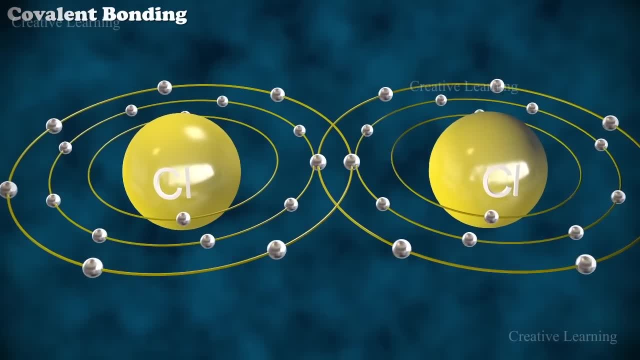 pair of electrons between the two chlorine atoms, each chlorine atom contributing one electron to the shared pair. Forty Buddhist Lab. The difference between electrons is in the gerekildrin barrier equation. The electron capsules are formed with 8 atoms within the second pair of electrons. 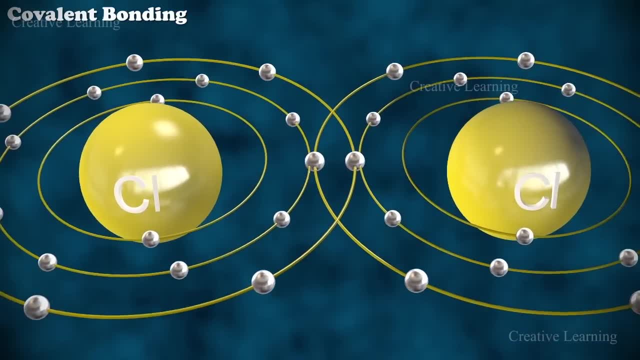 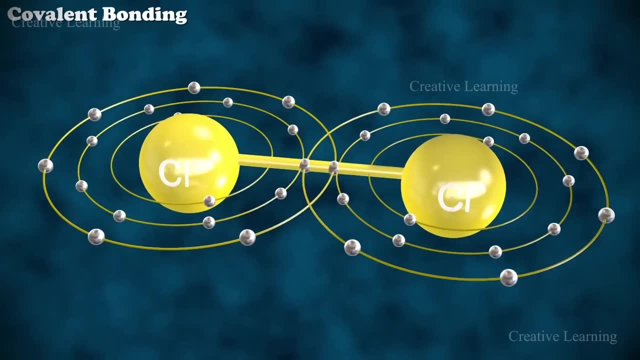 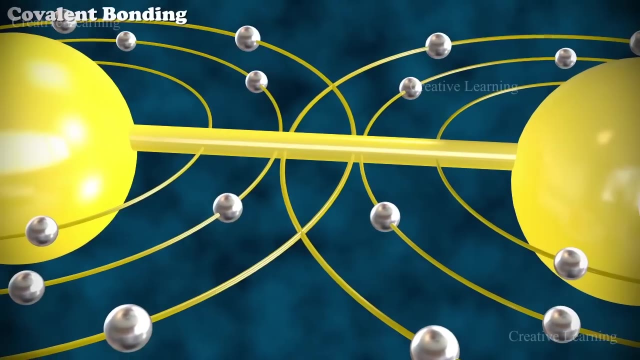 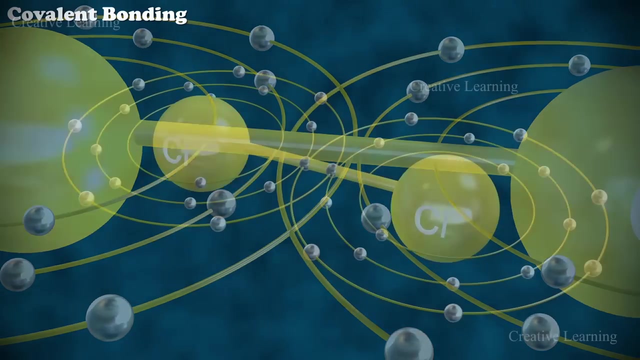 The bicarobronium atom is one electron. short of the argon configuration process, both chlorine atoms attain the outer shell octet of the nearest noble gas, that is, arcane. the dots represent electrons. such structures are referred to as Lewis dot structures. thus the chlorine atoms are joined by a single covalent bond. a single covalent bond is formed when one